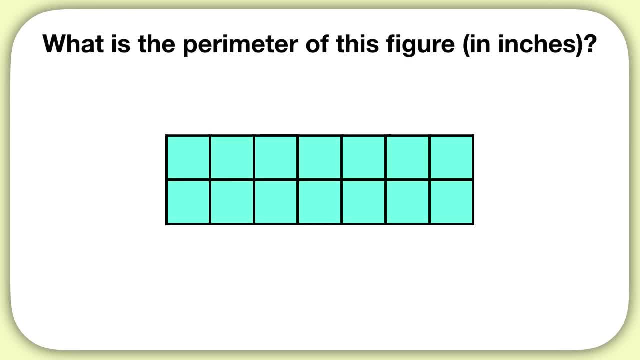 Let's look at one of these problems together. What is the perimeter of this figure in inches? Well, how do I find the perimeter of a shape? To find perimeter count the distance around the shape. Well, let's go ahead and do this. 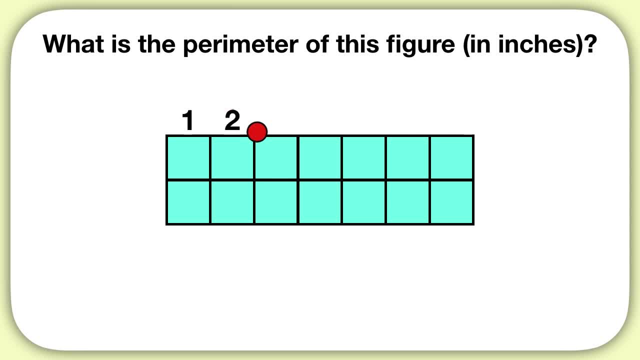 If I started here, I have to move 1,, 2,, 3,, 4,, 5,, 6, 7, then I move 8, 9 spaces. Now I want you to continue what I was just doing on your own. How far would you have to move to get around this? 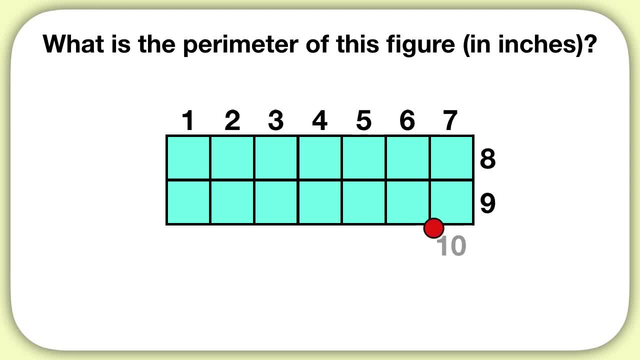 entire shape. Well, you can do that by counting the distance around the shape. So let's say you have to move 10,, 11,, 12,, 13,, 14,, 15,, 16,, 17,, 18 spaces, So we'll say the perimeter of this shape. 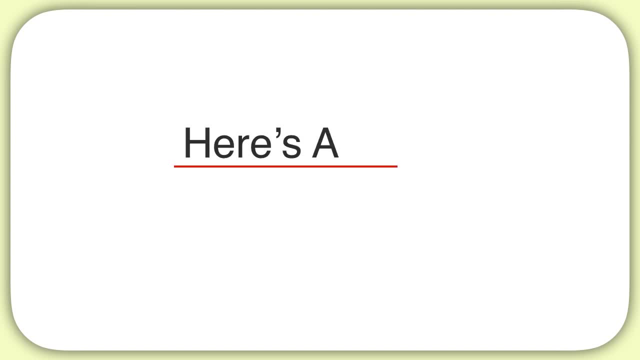 is 18 inches. Here's another problem to practice with: What's the perimeter of this figure in inches? Well, again, how do we find the perimeter of a shape? We count the distance around the shape to find perimeter. So if I start here and I move over here, how far did I just go? Well, 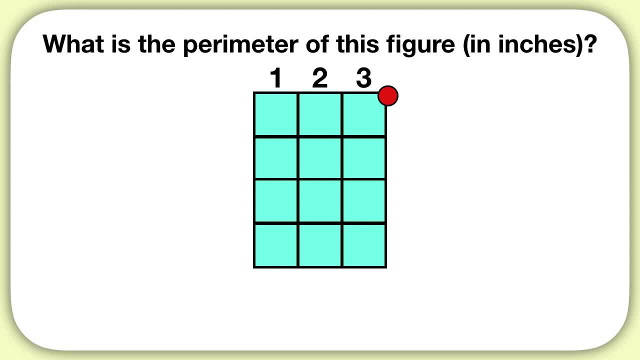 I just traveled 1 space, 2 spaces, 3 spaces. Then I move down here. Now I've gone 4,, 5,, 6,, 7 spaces, Then I can move over here. Now I've gone 8,, 9,, 10 spaces, And then I can move back. 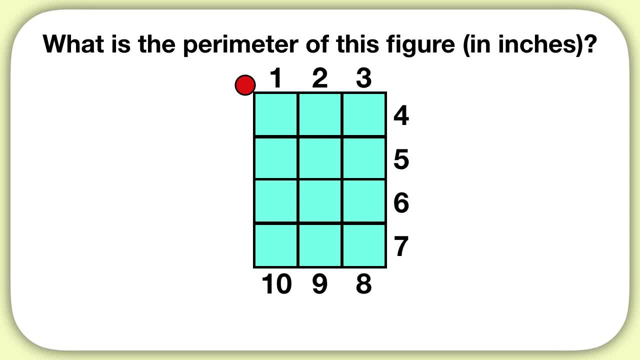 to where I started. How far will I have gone in total now? Well, I've gone 11,, 12,, 13,, 14 spaces. So the perimeter of this shape is 14 inches. Now it's time for you to practice. 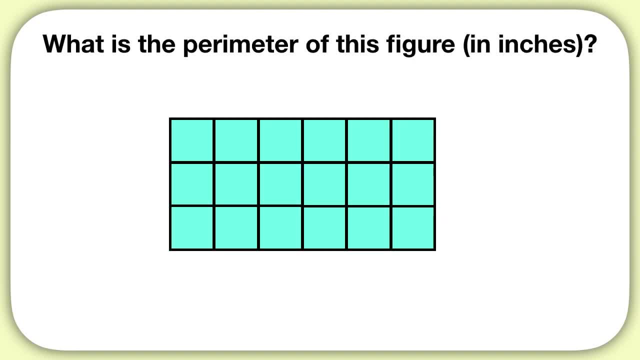 Practice on your own. What is the perimeter of this figure in inches? Well, think about starting here and you'll move 6 spaces, 7,, 8,, 9,, 10,, 11,, 12,, 13,, 14,, 15 spaces, 16,, 17,, 18.. And if you? 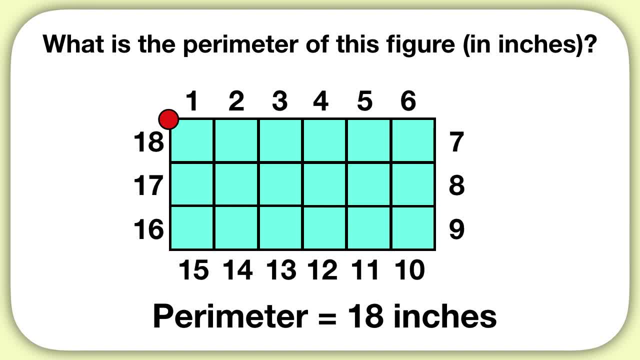 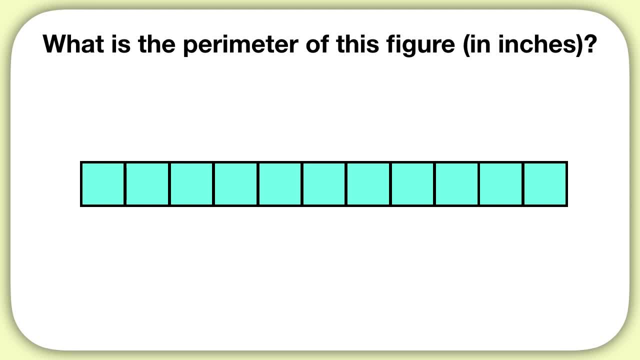 counted correctly, you'll get a perimeter of 18 inches. Now here's your last problem for this video. What is the perimeter of this figure? Well, if we start right here, we'll have to travel 11 spaces to get there, then 12, then all the way back to 23.. And now we've traveled a total of 24. 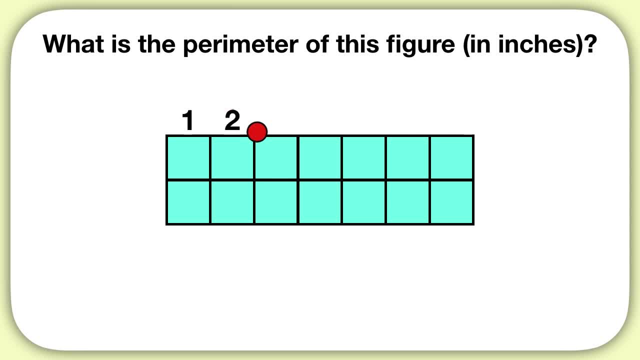 If I started here, I have to move 1,, 2,, 3,, 4,, 5,, 6, 7, then I move 8, 9 spaces. Now I want you to continue what I was just doing on your own. How far would you have to move to get around this? 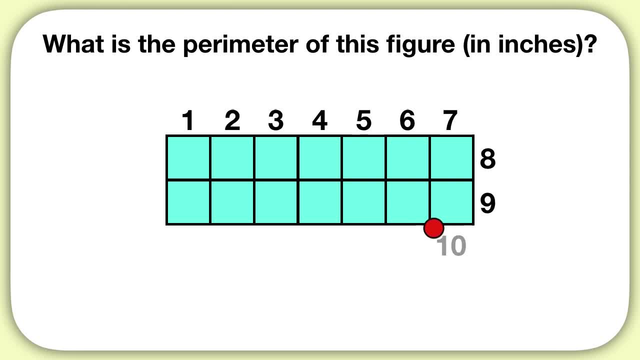 entire shape. Well, you can do that by counting the distance around the shape. So let's say you count it and move it at 커 slim deservedly. the circle around the top of the shape is 11 inches. What's the perimeter over here? Well, let's say you've got the perimeter and you. 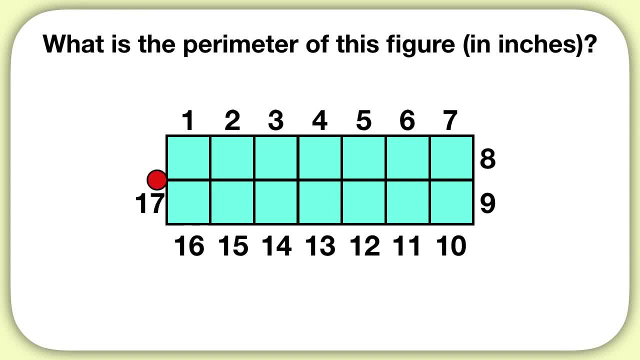 have to grab the edge of the shape. this is the présential, and you take the margin of two hundreds of inches and you take that còn to your right is your approximate. So now you would have to move 10,, 11,, 12,, 13,, 14,, 15,, 16,, 17,, 18 spaces, So we'll say the perimeter. 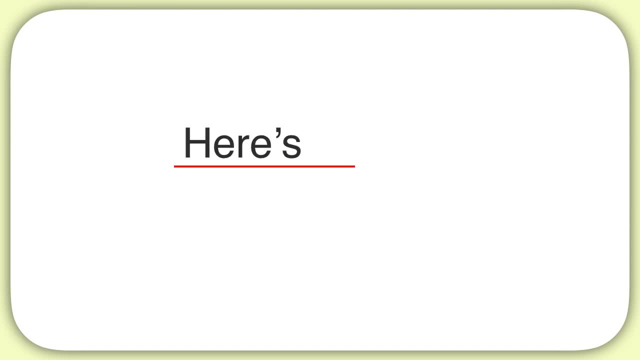 of this shape is 18 inches. Well, that's how you do it. so now we're going to see how long it'd take you to take the entire shape. Here's another problem to practice with: What's the perimeter of this figure in inches? Well, again, how do we find the perimeter of a shape? 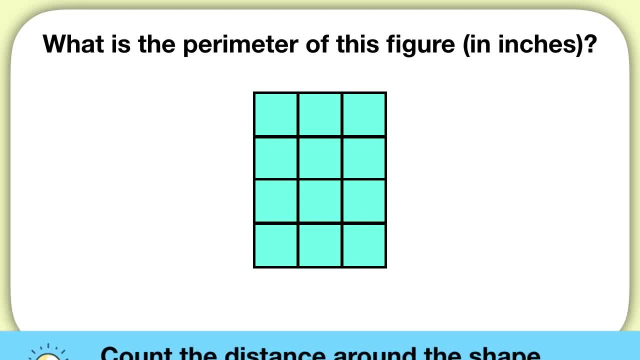 We count the distance around the shape to find perimeter. So if I start here and move over here, how far did I just go? I just traveled one space, two spaces, three spaces, Then I move down here. Now I've gone four, five, six, seven spaces, Then I can move over here. 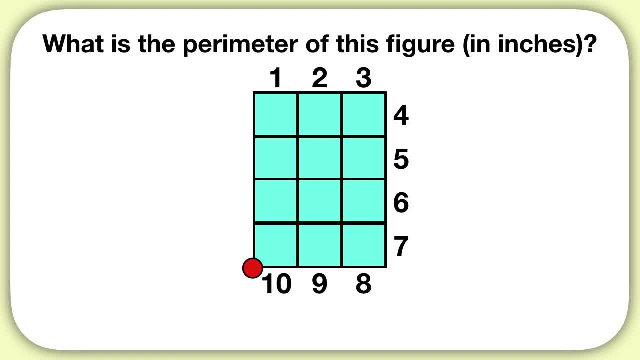 Now I've gone eight, nine, ten spaces, And then I can move back to where I started. How far will I have gone in total now? Well, I've gone 11,, 12,, 13,, 14 spaces. So the perimeter. 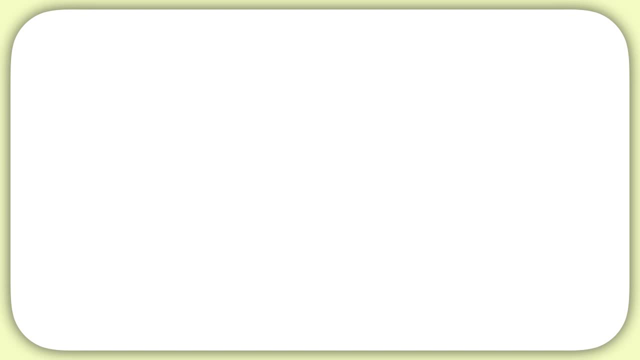 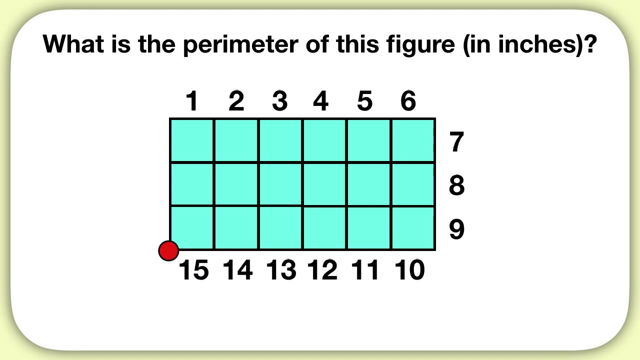 of this shape is 14 inches. Now it's time for you to practice on your own What is the perimeter of this figure in inches? Well, think about starting here and you'll move six spaces, seven, eight, nine, 10,, 11,, 12,, 13,, 14,, 15 spaces, 16,, 17,, 18.. And if you, 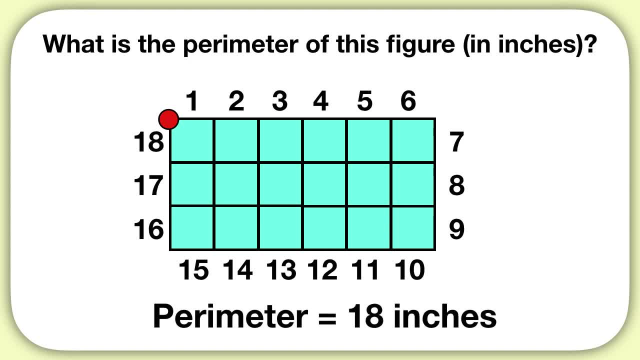 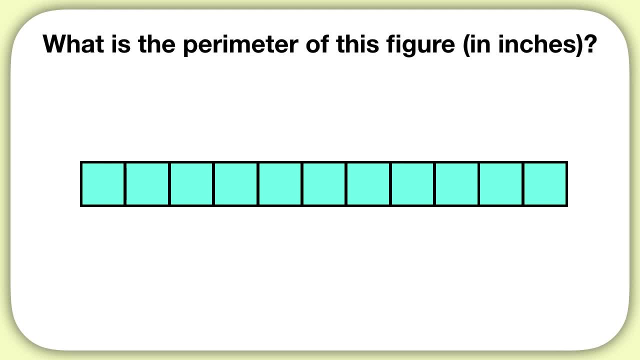 counted correctly, you'll get a perimeter of 18 inches. Now here's your last problem for this video. What is the perimeter of this figure in inches? Well, the perimeter of this figure in inches is the perimeter of this figure. Well, if we start right here, we'll have to travel. 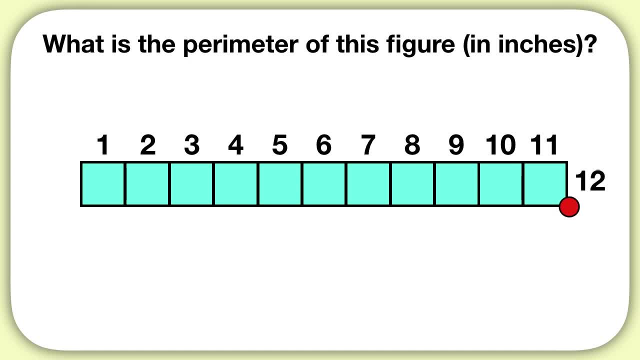 11 spaces to get there, then 12, then all the way back to 23.. And now we've traveled a total of 24 spaces. So the perimeter of this shape is 24 inches. Today you learned how to find perimeter by counting distance.